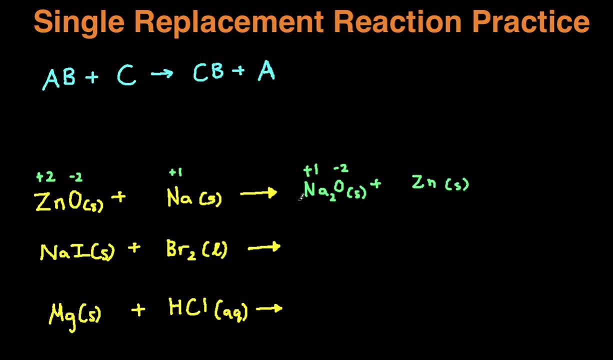 it's going to be solid as well. Then we double check if the reaction is balanced. You can see here there's two sodiums, so I'm going to need two in front of the sodium on the reactant side to make that balance. And then, after doing that, 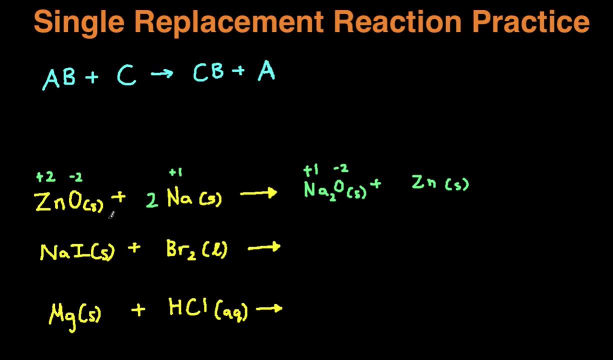 the entire reaction is balanced. Great, let's go and do the second example. Again, we have an ionic compound reacting with a compound made up of a single element. so this is going to be a single replacement reaction. We're going to write the charges: sodium, first column, so it's positive one. 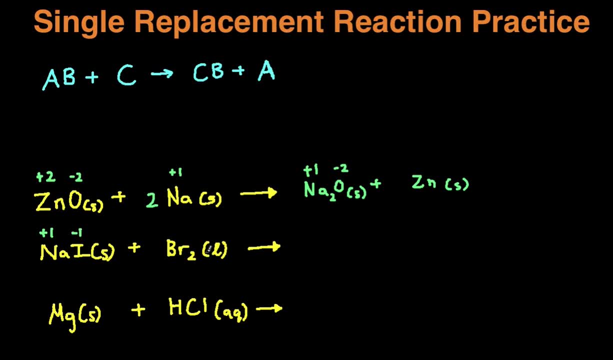 iodine, because it's a halogen, it's negative one. and then bromine. if it were to be an ionic compound, since it's a halogen, it would also be negative one. Now the element has a negative charge, unlike the element on top, which has positive charge. so now we're going to 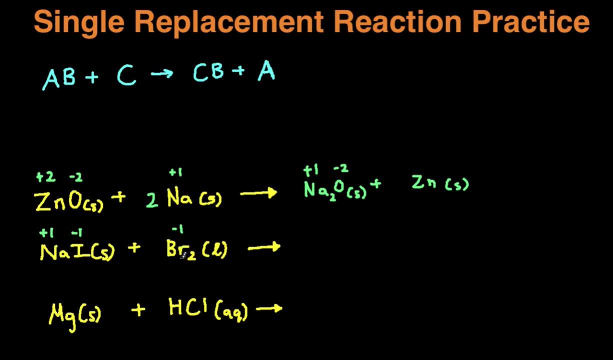 take. we're going to switch. the two elements are negatively charged, so we're going to switch the Br and I, and then that's going to give us Na Br. and I Notice, although there was two Brs here, I only brought one Br over to the other side, and the reason why I did that is because I want to. 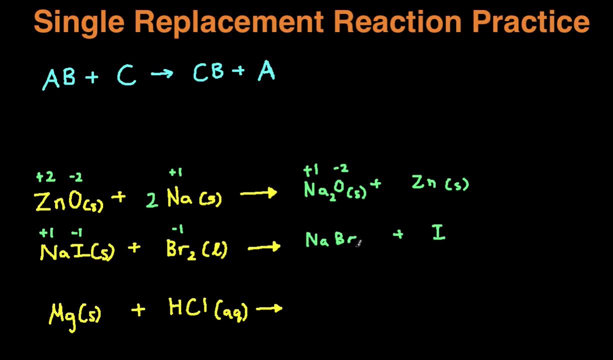 make sure the charges are balanced before I add subscripts. So now I carried the charges over, sodium is positive one and then bromine is negative one, so you can see these currently do balance each other out, so I don't there's no need to add any more subscripts. 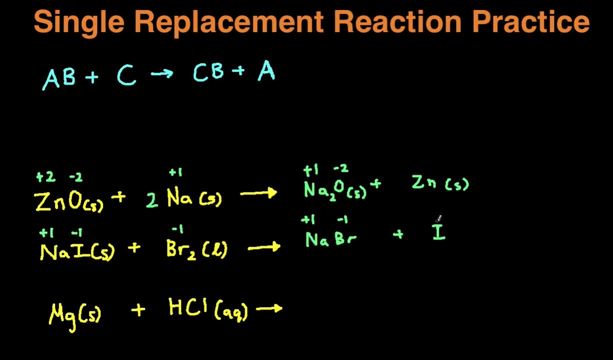 Now iodine in, since it is a diatomic element. when iodine is alone, it's going to be in a pair. so I2 and iodine in standard state is going to be in salt, a solid, and then sodium bromide- because it is an ionic compound, it's also going to be a solid. Then we double check if the iodine is. 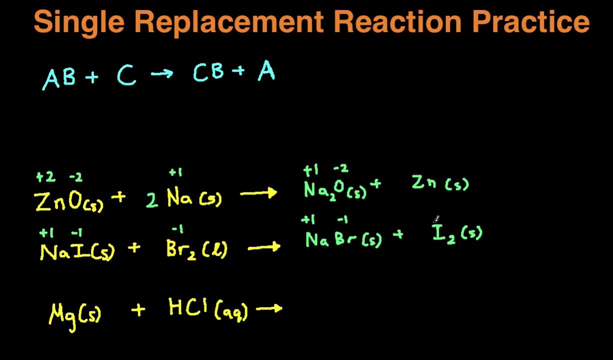 balanced I. there's currently two I's on the reactant side and only one on the- I mean sorry, the two on the product side and one on the reactant side. so I'm going to need a two right here and then that makes this. I have two sodiums. I need to put a two in front of here and then after. 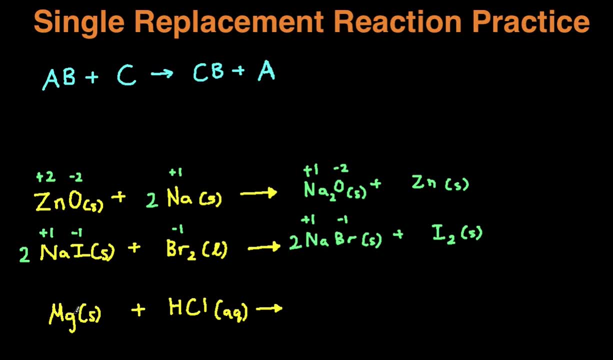 doing that, everything is balanced, Okay. last example: we have magnesium reacting of hydrochloric acid. so we have a metal reacting with a ionic like substance as hydrochloric acid, since this is a strong acid. so again, this is going to be single replacement. then we're going to write the charges.